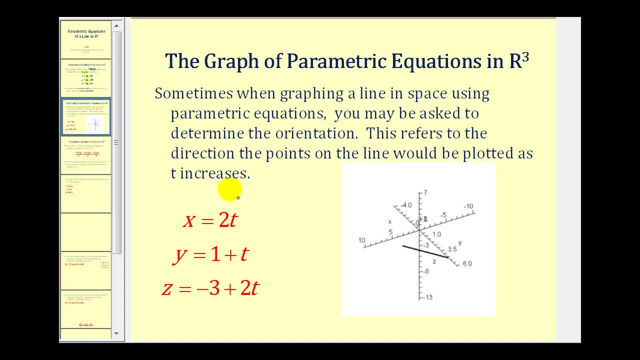 the points on the line would be plotted as t increases. So here's the graph of the line defined by: x equals 2t, y equals 1 plus t and z equals negative 3 plus 2t. We can see that as: 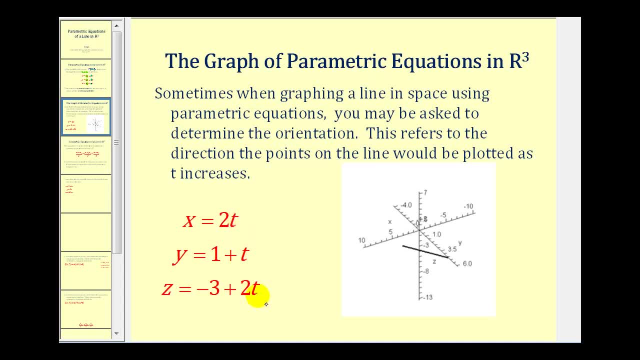 t increases, all three of these coordinates will also increase, because the coefficients of all of the t terms are positive. More specifically, as t increases, so does z, And you can think of z as the height of the line. So as t increases, this line is moving upward. So we know the orientation. 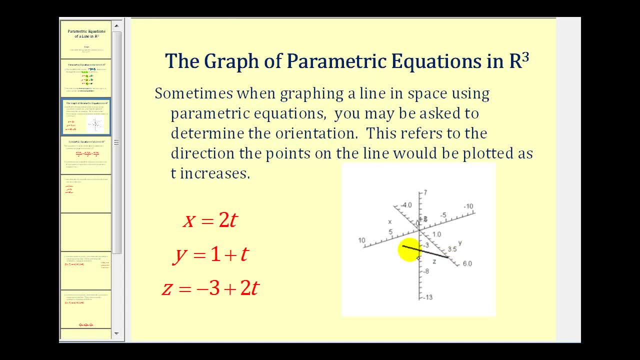 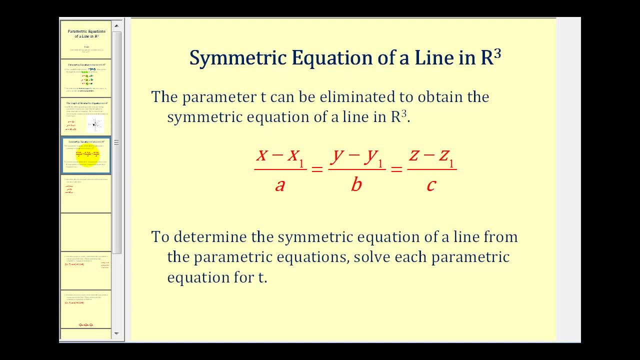 of this line would be from this direction to the left or in this direction. here There's one more form of a linear equation we should mention for r3.. The parameter t can be eliminated to obtain what's called the symmetric equation of a line in r3. So this form of a line in space is a symmetric equation of a line. To obtain this, 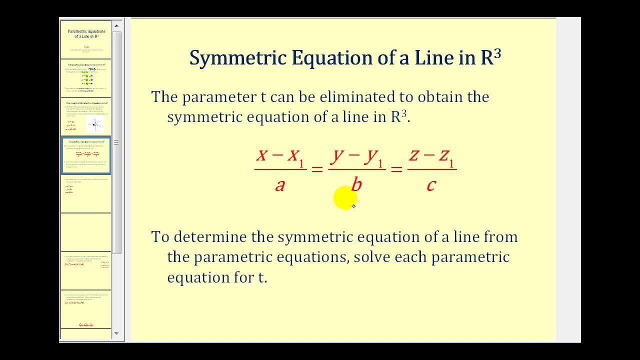 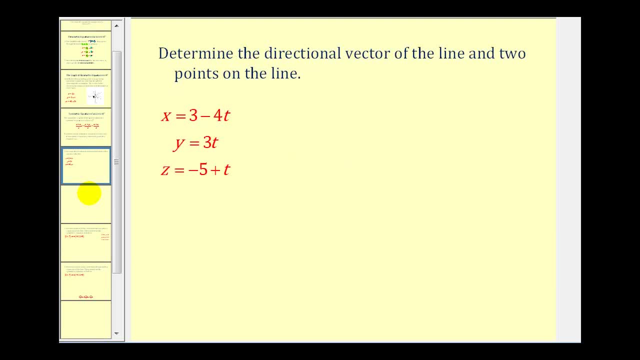 what we can do is solve each equation for t and then set them all equal to each other. Let's go and take a look at an example. Here we want to determine the directional vector of the line and two points on the line. Remember, the directional vector for the line is determined by 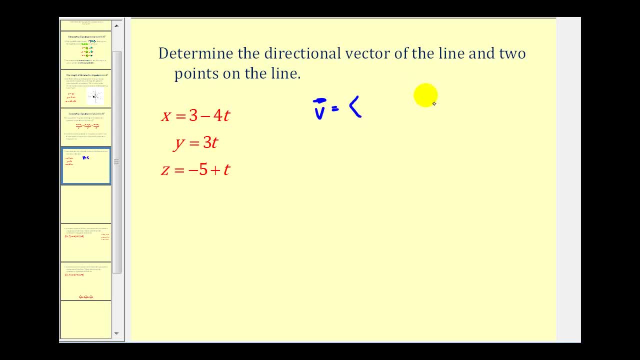 by the coefficients of the t terms. So the directional vector would have components negative four, positive three and positive one. Now let's try to find two points on the line. We can find the first point. we'll call it point P. 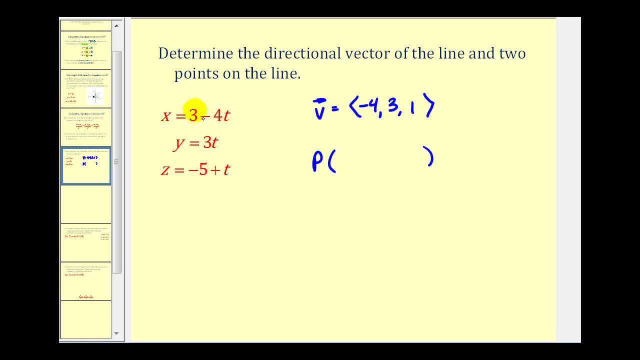 by the constants of each of these equations. So the x coordinate would be positive three, the y coordinate would have to be zero and the z coordinate would be negative five. But they ask for two points on the line. so to determine one more point on the line, 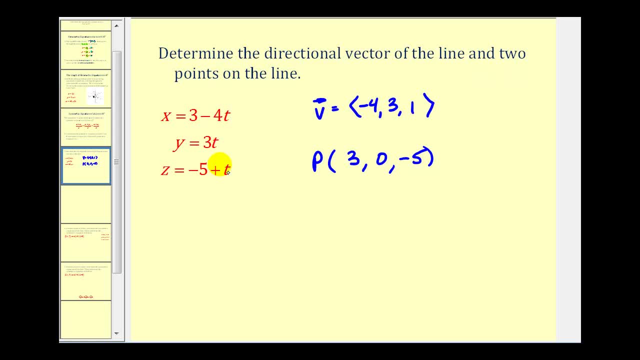 we'll have to select a value for t and sub it into each of these equations. So for the second point, let's call it q. If we let t equal zero, we're going to come up with the same point that we just found. 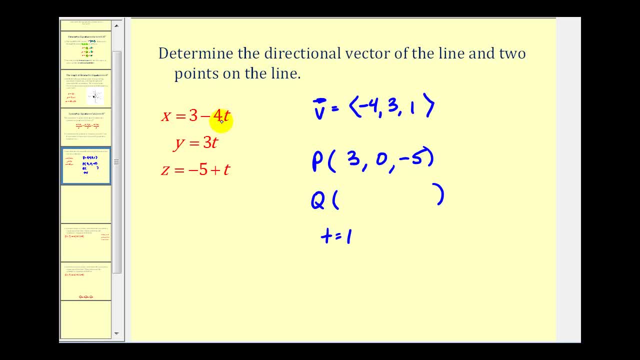 So let's go ahead and let t equal one. So if t is equal to one, we'd have three minus four. so that would be negative one for the x coordinate, positive three for the y coordinate, and then for z we'd have negative five plus one. 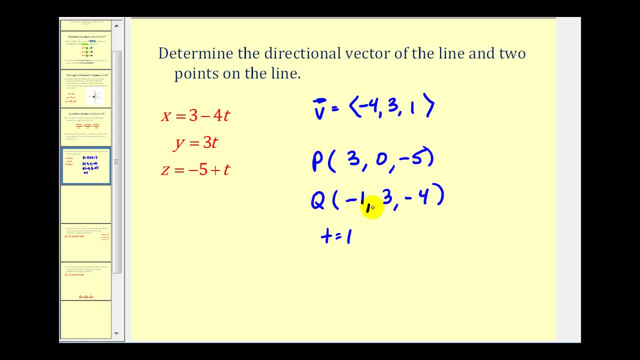 that would give us negative four. Now, remember, there's an infinite number of points on a line, but these are just two points that are pretty convenient to find. Let's go and take a look at the graph of this line. Here it is in red, and again, if we rotate, 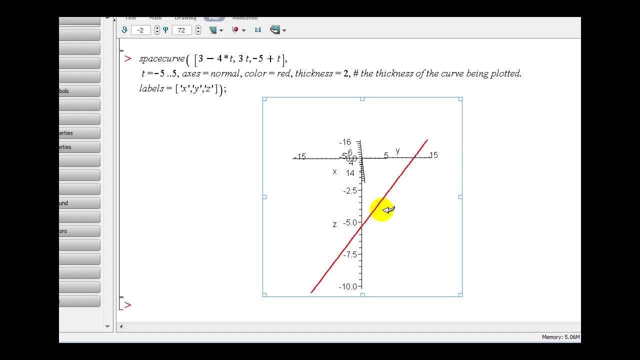 this coordinate system we get a better idea of the line's orientation in space. Notice: the line is below the x- y plane until t is greater than positive five. So the orientation of this line would be from left to right as t increases. 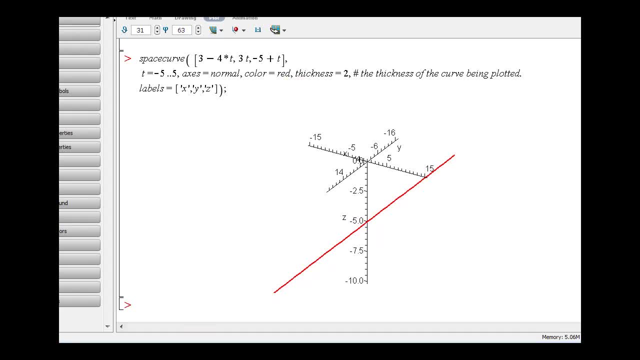 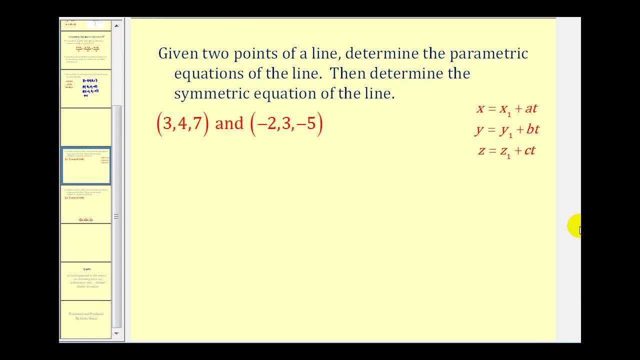 Let's go and take a look at another example. Here we're given two points on a line. We want to determine the parametric equation of the line and then also determine the symmetric equation of the line. So, looking at the parametric equations of a line, 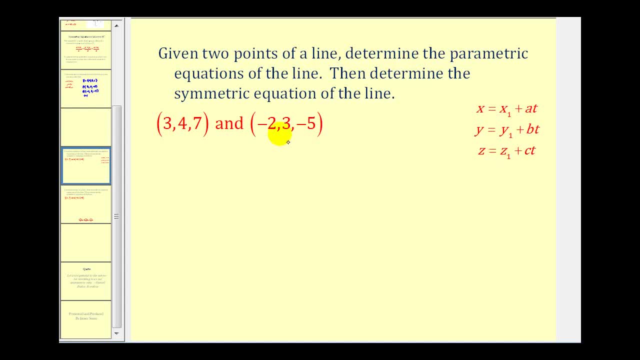 we're going to have two points on a line. We can let either of these points represent x sub one, y sub one and z sub one, But remember to find the values of a, b and c we have to find the directional vector of this line. 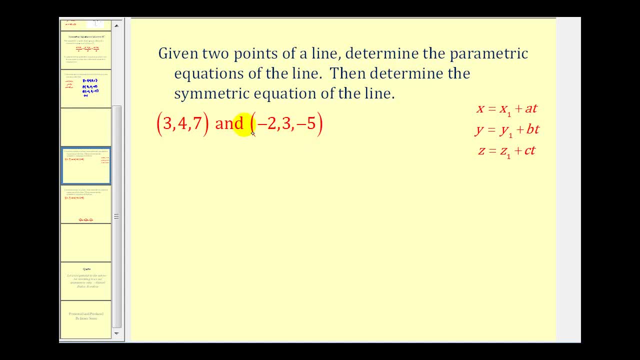 And we can do that by finding the vector in component form that would pass through these two points. So we'll call our directional vector vector v, where the x component will be negative two minus three, The y coordinate will be positive three minus four. 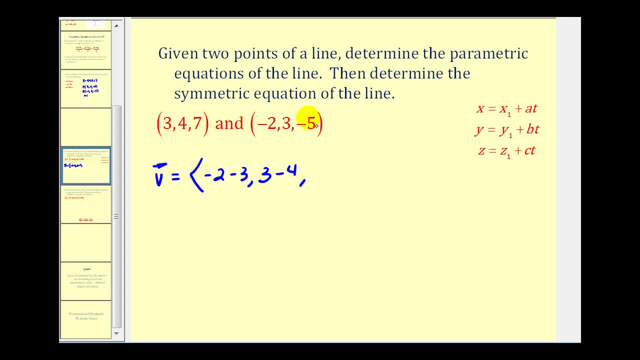 And the z component will be negative five minus seven. So our directional vector, which will give us a, b and c, will be negative five, negative one and negative 12.. And again, we'll go ahead and use the first point. 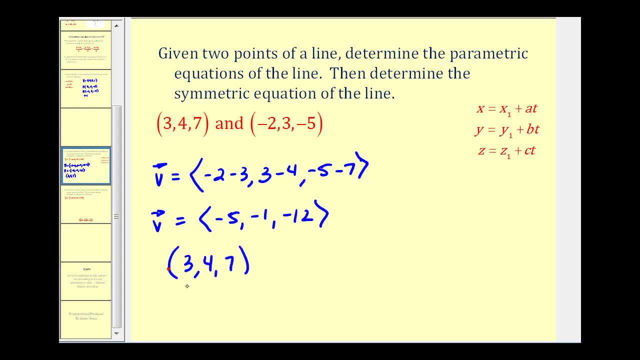 three, four, seven, to represent x sub one, y sub one and z sub one. But we could use any other point on the line if we wanted to, So the parametric equations of the line passing through these two points will be: